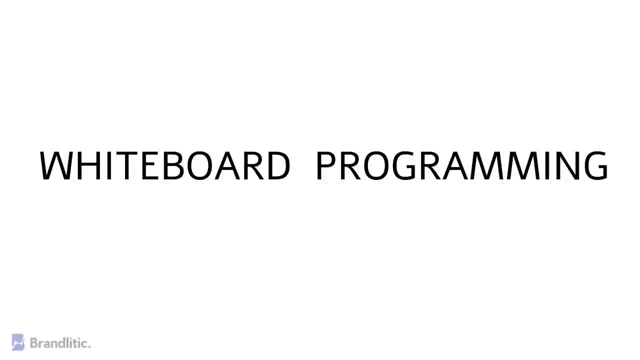 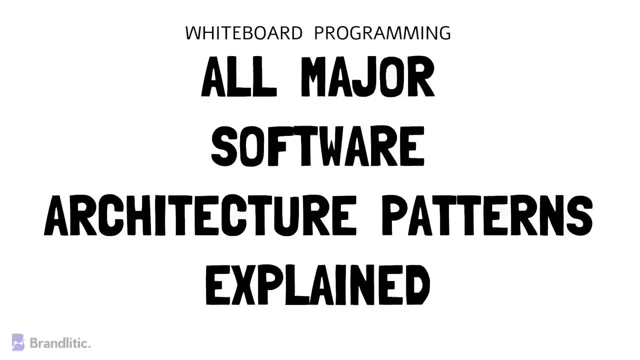 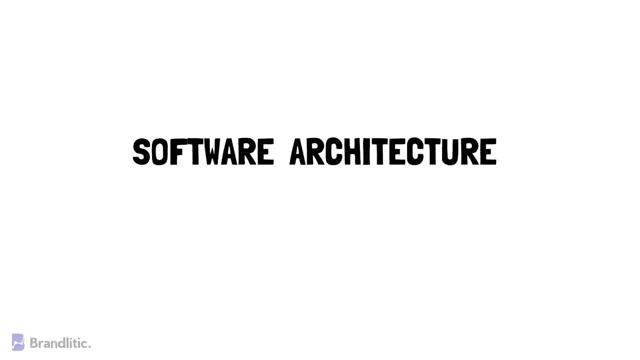 Welcome to Web-Bed Programming, where we simplify programming with easy to understand whiteboard videos, and today I'll be sharing with you the most common software architecture patterns that are used by enterprises all across the globe. So let's get started. First, as basics, let me briefly explain what is a software architecture. Well, it is nothing. 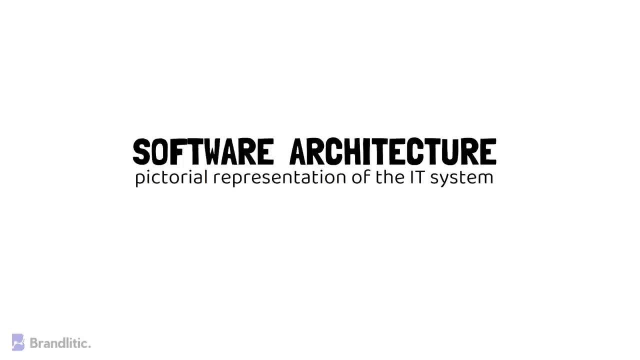 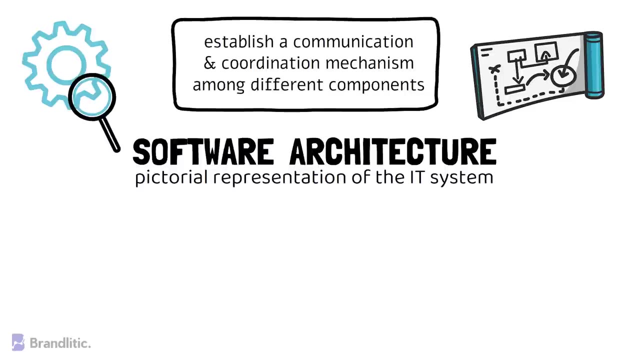 but a pictorial representation of the IT system that serves as a blueprint for a system. It provides an abstraction to manage the system complexity and establish a communication and coordination mechanism among different components in it. It also helps define a structured solution to meet all the technical and operational requirements while optimizing the common 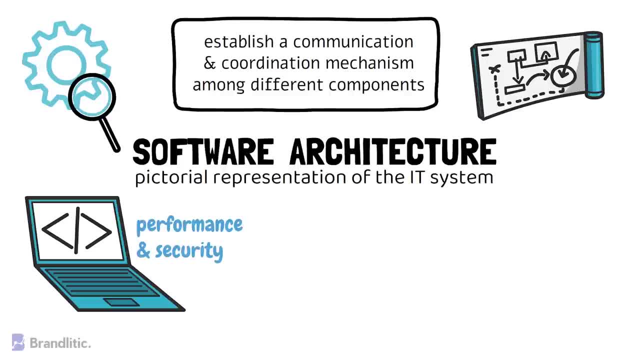 quality attributes like performance and security. The primary goal of a software architecture is to identify requirements that affect the structure of the application. A well-laid architecture reduces the business risks associated with building a technical solution and builds a bridge between business and technical requirements. 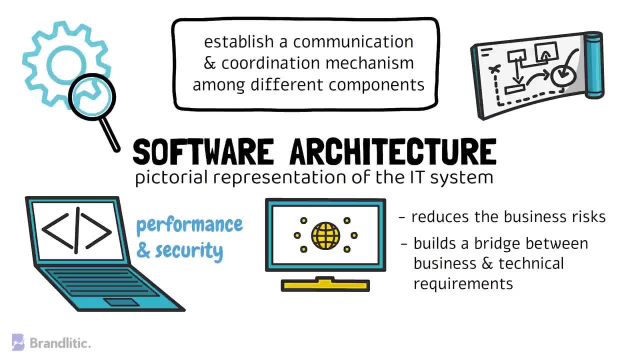 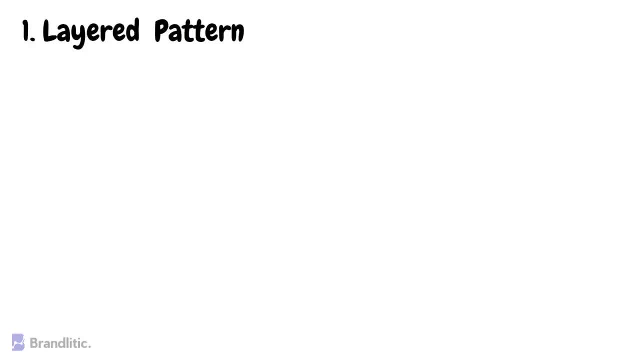 With that being said, let's start understanding major software architecture patterns, starting with 1. Layered Pattern. This pattern can be used to structure programs that can be decomposed into groups of subtasks, each of which is at a particular level of abstraction. Here, each layer provides services to the next higher layer. 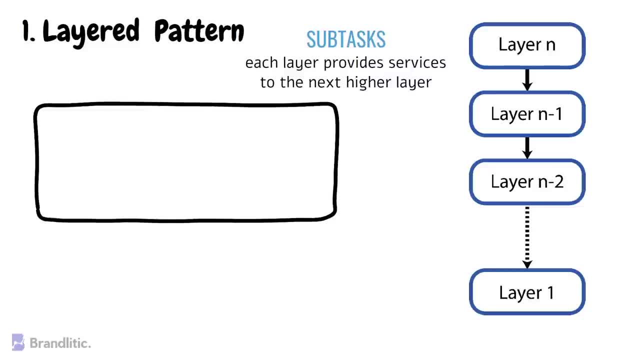 The most commonly found four layers of a general information system are as follows: 1. Presentation Layer. 2. Application Layer. 3. Business Logic Layer. 4. Data Access Layer. 5. Persistent Layer. Such a setting of software architecture is widely used in building general desktop applications. 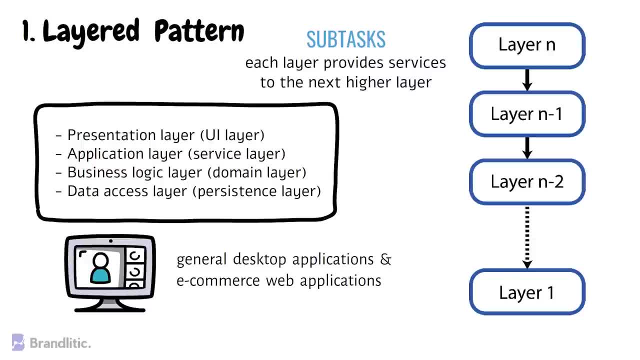 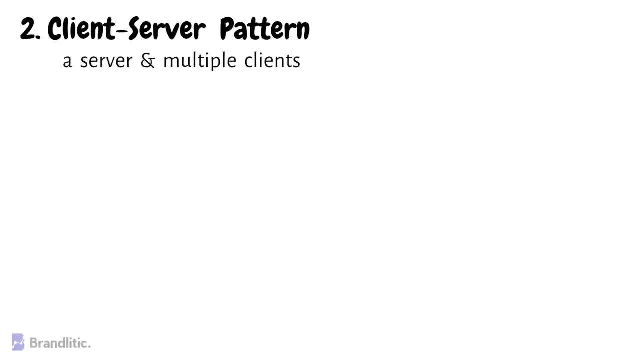 and e-commerce web applications. 2. Client-Server Pattern. This pattern consists of two parties: a server and multiple clients. Here the server component will provide services to multiple client components. Client requests services from the server and the server provides relevant services. 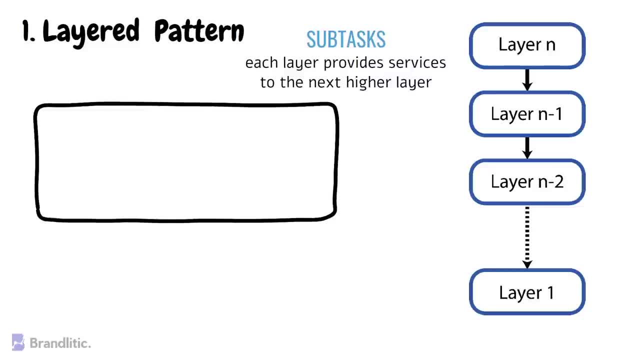 The most commonly found four layers of a general information system are as follows: 1. Presentation Layer. 2. Application Layer. 3. Business Logic Layer. 4. Data Access Layer. 5. Persistent Layer. Such a setting of software architecture is widely used in building general desktop applications. 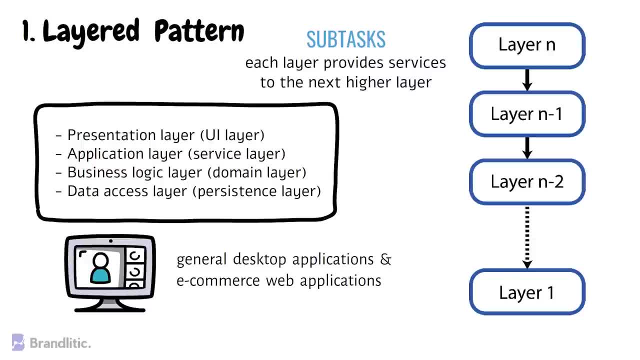 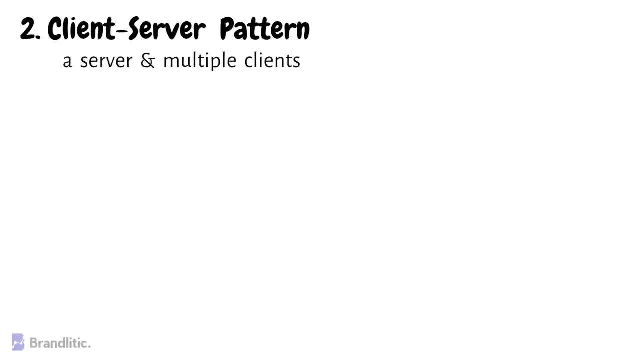 and e-commerce web applications. 2. Client-Server Pattern. This pattern consists of two parties: a server and multiple clients. Here the server component will provide services to multiple client components. Client requests services from the server and the server provides relevant services. 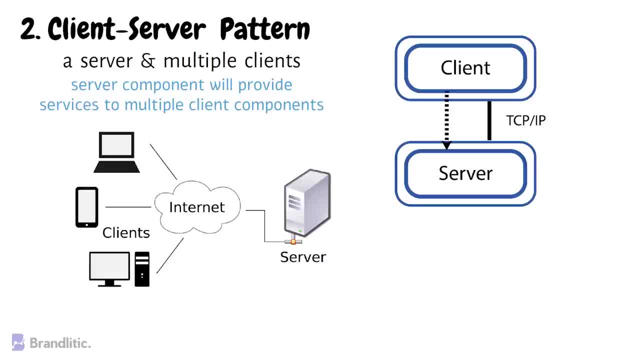 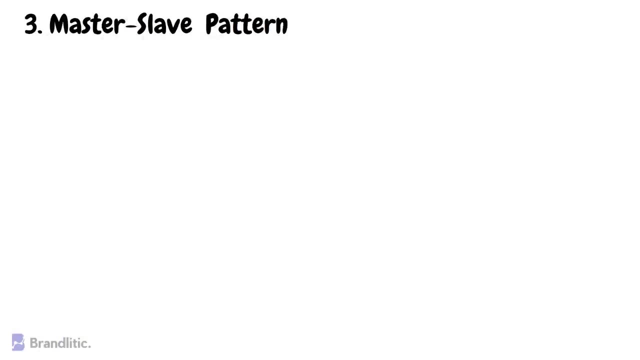 to those clients. Furthermore, the server continues to listen to the client requests as well. This software architecture is generally used in online applications such as email, document sharing and banking, etc. 3. Master-Slave Pattern. This pattern consists of two parties. 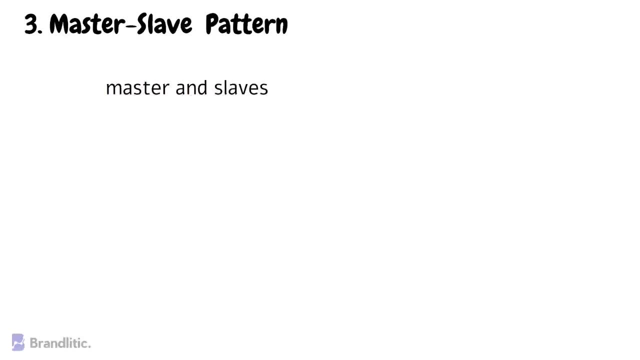 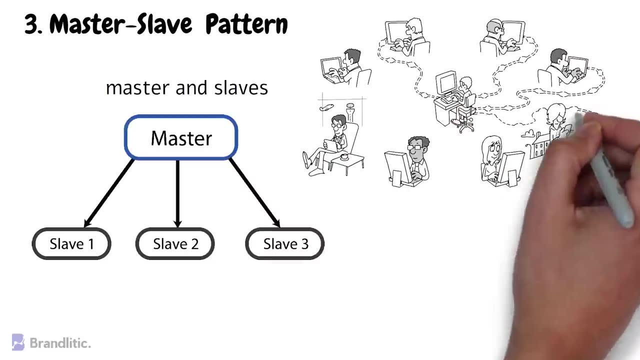 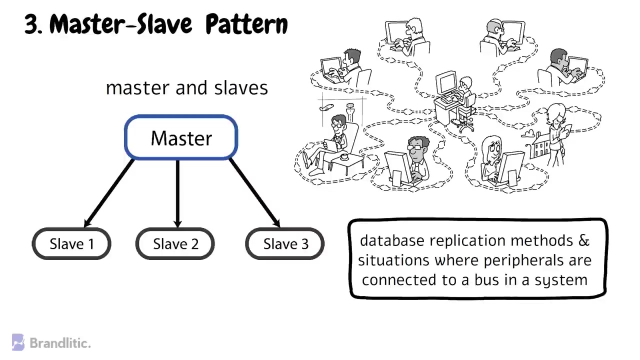 master and slave. Here the master component distributes the work among identical slave components and computes a final result from the results which the slaves return. This architecture pattern is employed in database application methods and situations where peripherals are connected to a bus in the system. 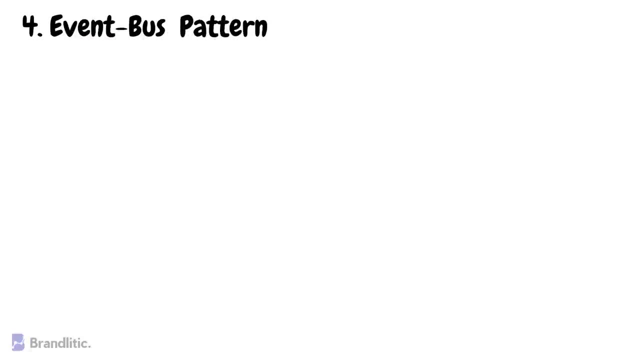 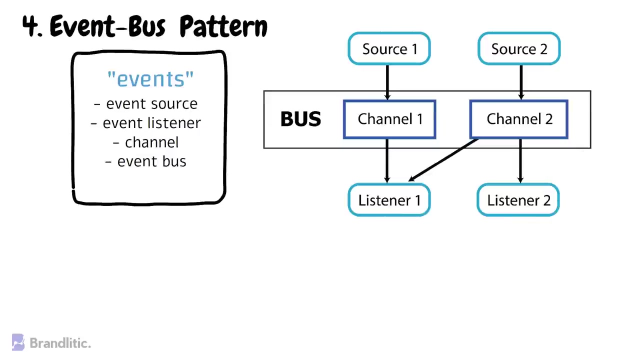 4. Event Bus Pattern. This pattern primarily deals with events and has four major components: event source, event listeners channel and event bus. Here the source publishes messages to a particular channel on the event bus and listeners subscribe to that particular channel. Therefore listeners are notified of. 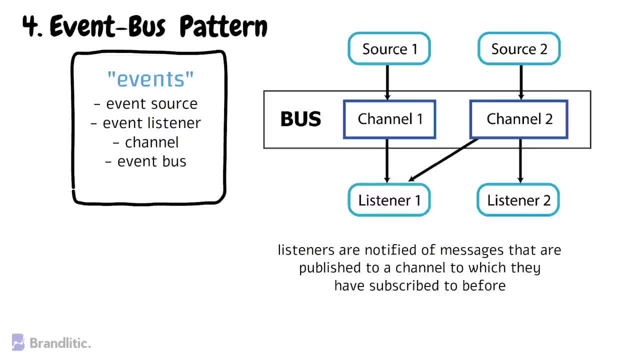 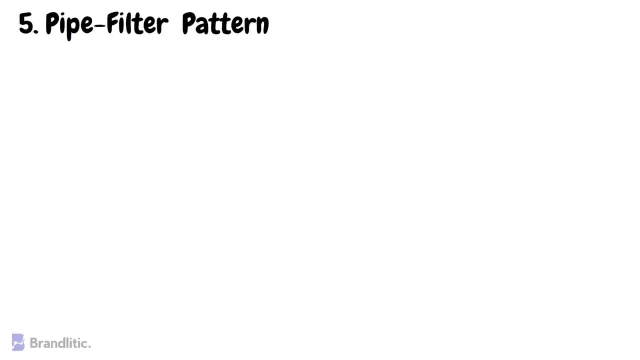 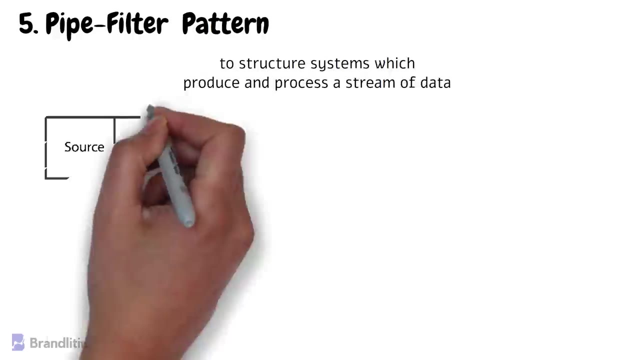 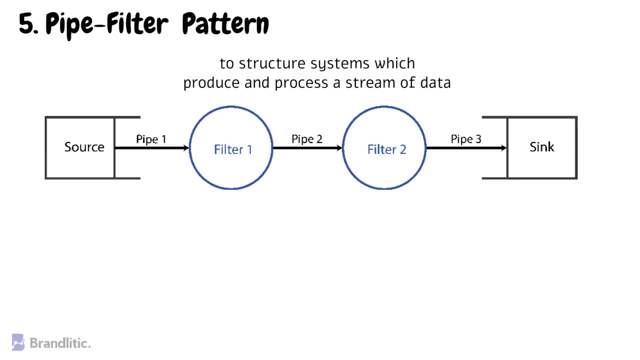 messages that are published to a channel to which they have subscribed. 5. Pipe Filter Pattern. This pattern can be used to structure systems which produce and process a stream of data. Here, each processing step is enclosed within a filter component. Data to be processed is passed through pipes, and these pipes can be used for buffering. 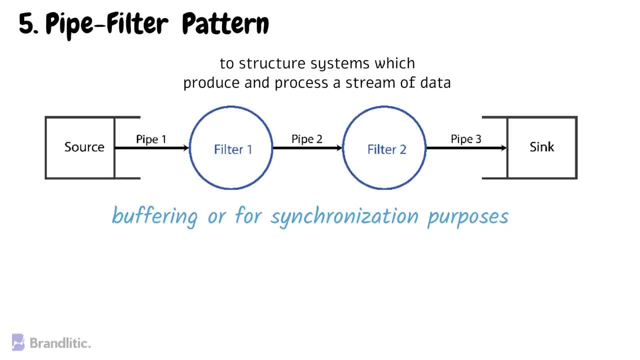 or for synchronization purposes. Here each processing step is enclosed within a filter. Here each processing step is enclosed within a filter. Here each processing step is enclosed within a filter. This architecture pattern is used in building compilers and defining workflows in bioinformatics. 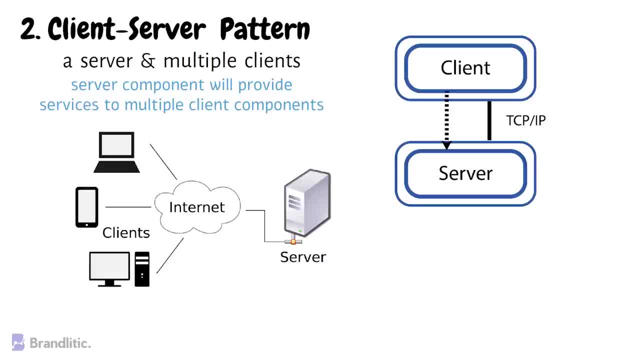 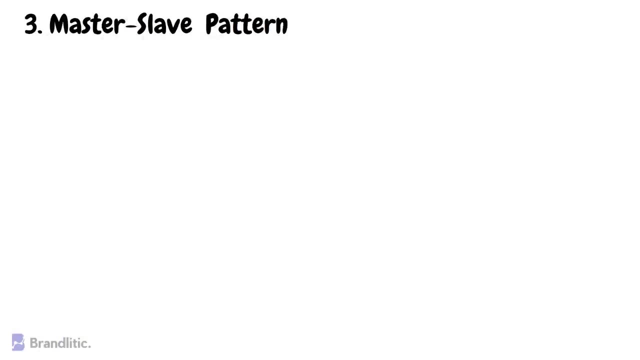 to those clients. Furthermore, the server continues to listen to the client requests as well. This software architecture is generally used in online applications such as email, document sharing and banking, etc. 3. Master-Slave Pattern. This pattern consists of two parties. 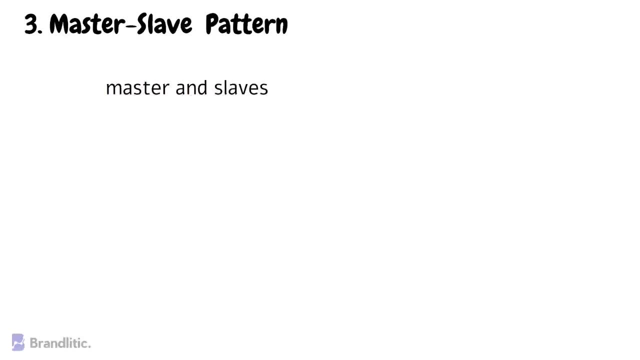 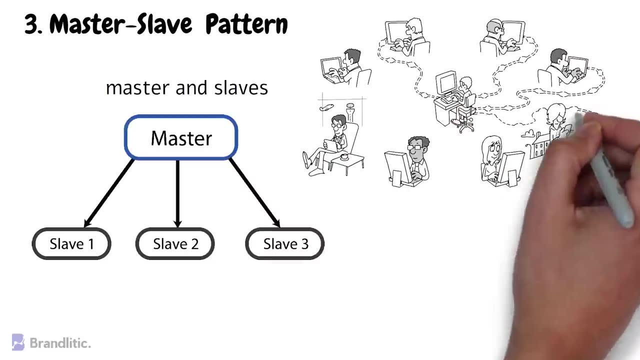 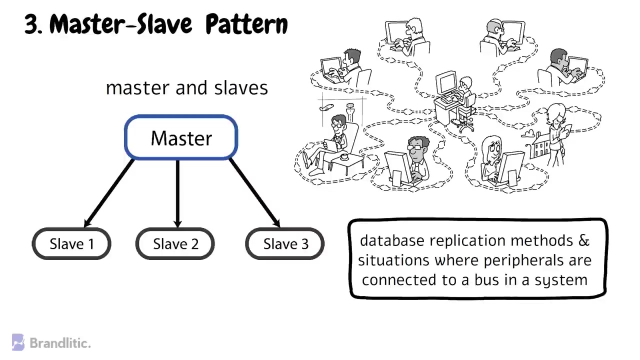 master and slave. Here the master component distributes the work among identical slave components and computes a final result from the results which the slaves return. This architecture pattern is employed in database application methods and situations where peripherals are connected to a bus in the system. 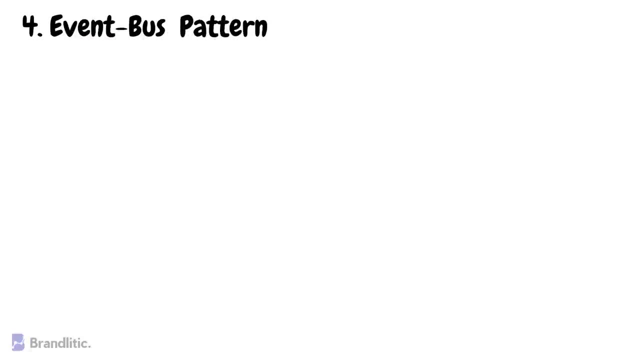 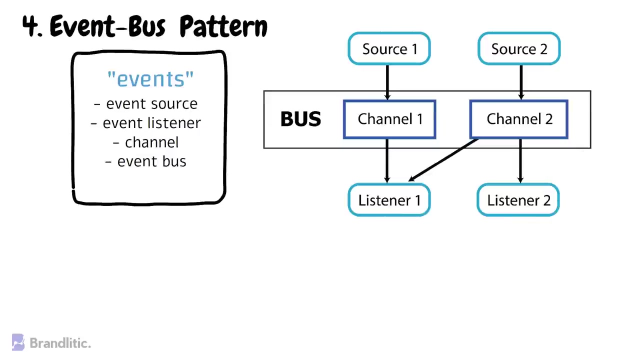 4. Event Bus Pattern. This pattern primarily deals with events and has four major components: event source, event listeners channel and event bus. Here the source publishes messages to a particular channel on the event bus and listeners subscribe to that particular channel. Therefore listeners are notified of. 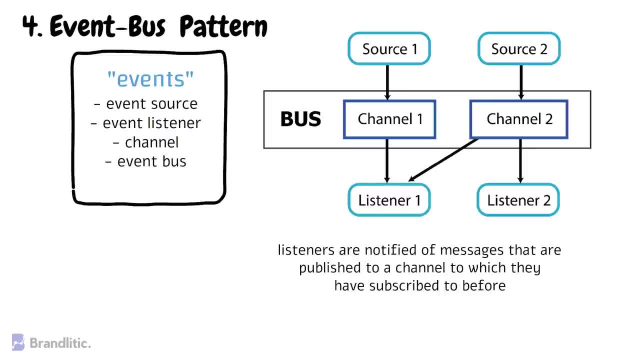 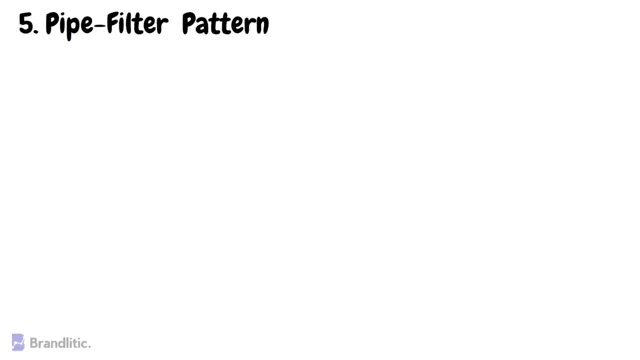 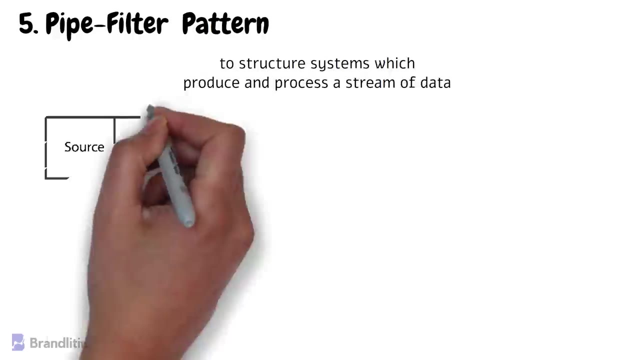 messages that are published to a channel to which they have subscribed. This software architecture pattern is used in Android Devel and is widely employed in building notification services. 5. Pipe Filter Pattern. This pattern can be used to structure systems which produce and process a stream of data. Here, each processing step is enclosed. 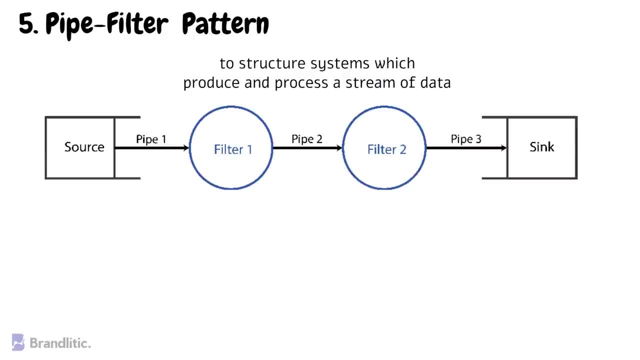 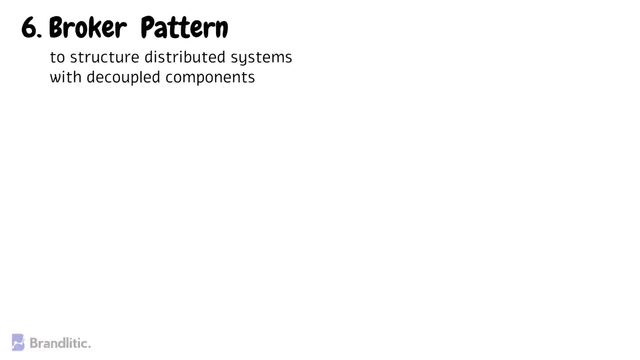 within a filter component, Data to be processed is passed through pipes, and these pipes can be used for both buffering and synchronization purposes. This architecture pattern is used in building compilers and defining workflows in bioinformatics. 6. Broker pattern: This pattern is used to structure distributed systems with decoupled components. 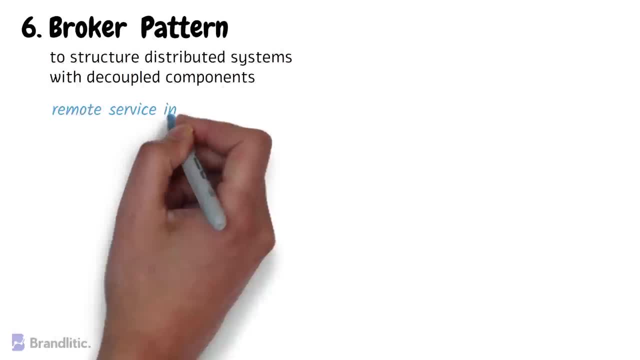 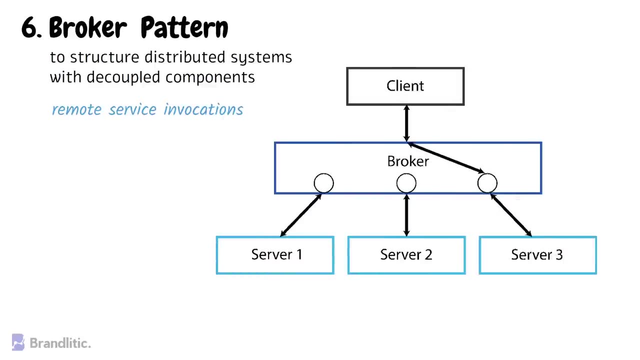 These components can interact with each other by remote service invocations, and a broker component is responsible for the coordination of communication among the components. Here servers publish their capabilities, which are services and characteristics to a broker, and clients request a service from the broker, and the broker then redirects the client to a suitable service from its registry. 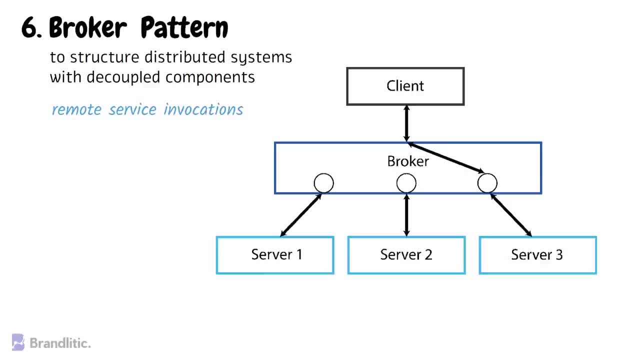 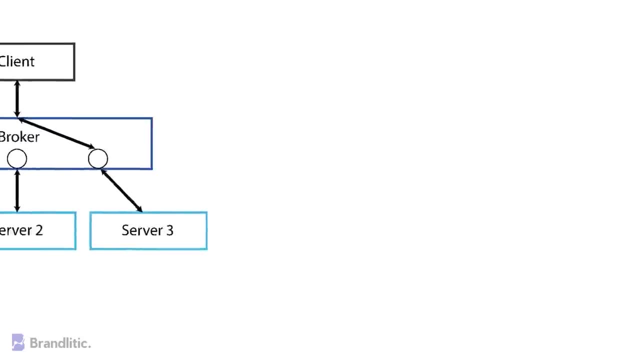 This particular architecture is generally employed in message broker software such as Apache, Kafka and JBoss messaging. 7. Peer-to-peer pattern. In this pattern, individual components are known as peers. Now do note that peers may function both as clients requesting services from other peers. 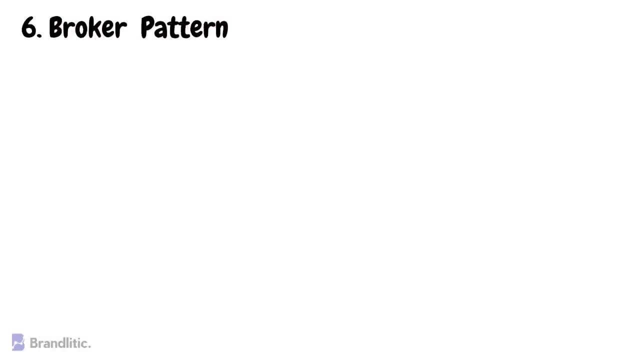 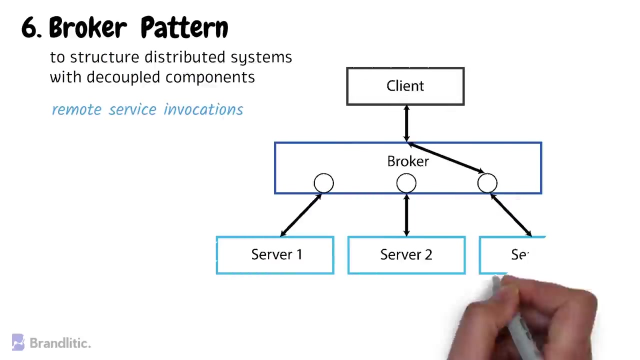 6. Broker Pattern. This pattern is used to structure distributed systems with decoupled components. These components can interact with each other by remote service invocations, and a broker component is responsible for the coordination of communication among the components. Here servers publish their capabilities, which are services and 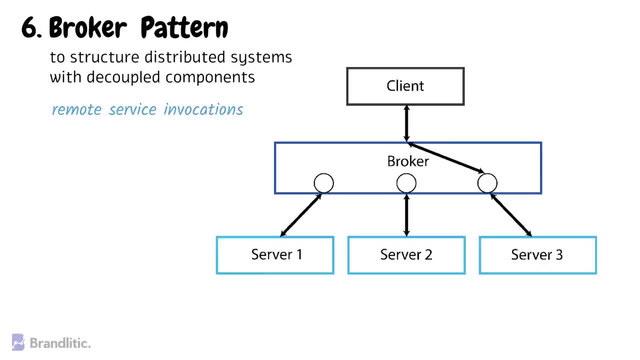 characteristics to a broker and clients request a service from the broker, and the broker then redirects the client to a suitable service from its registry. This particular architecture is generally employed in message broker software such as Apache, Kafka and JBoss Messaging. 7. Peer-to-Peer Pattern. In this pattern, individual components: 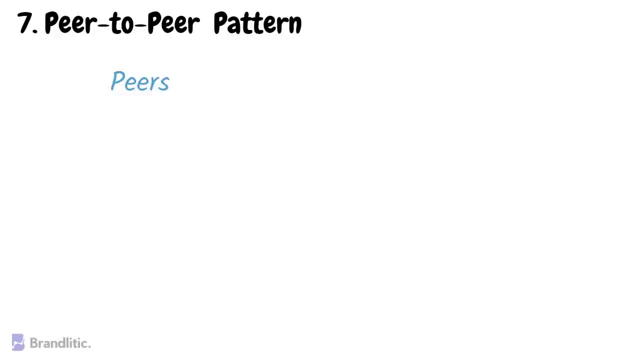 are known as peers. Now, do note that peers may function both as client, requesting services from other peers, or as servers providing services to other peers. A peer may act as a client or as a server, or as both, and it can change its role dynamically with time. It is widely 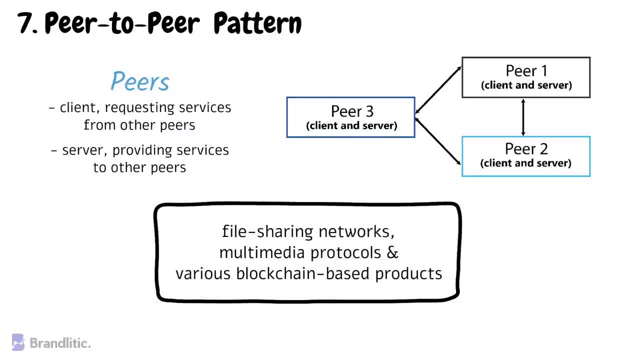 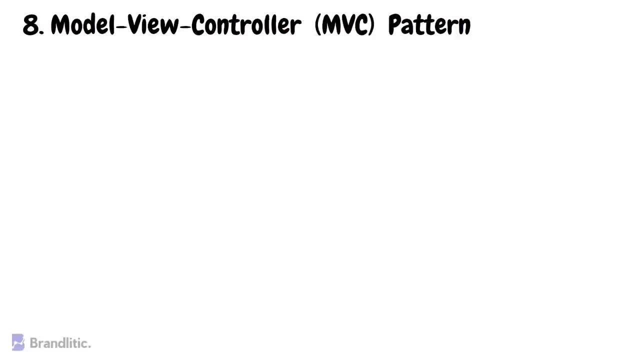 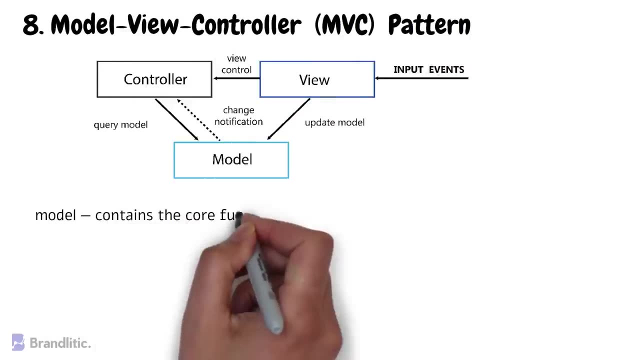 used in building file-sharing networks, multimedia protocols and various blockchain-based products. 8. Model-View-Controller Pattern. This pattern, also known as MVC pattern, divides an interactive application into three parts As: 1. Model, which contains the core functionality and data. 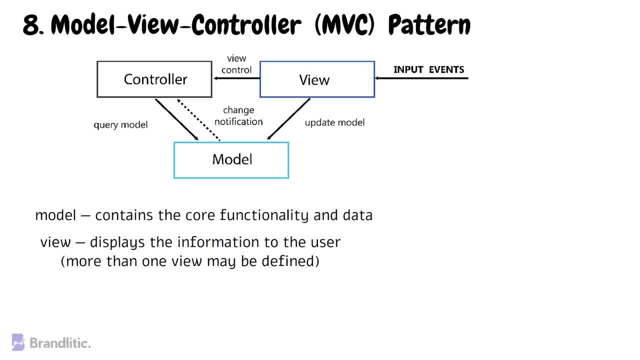 2. View which displays the information to the user, and more than one view may be defined as well. 3. Controller, which handles the input from the user. This is done to separate internal representations of information from the ways information is presented to and accepted from. 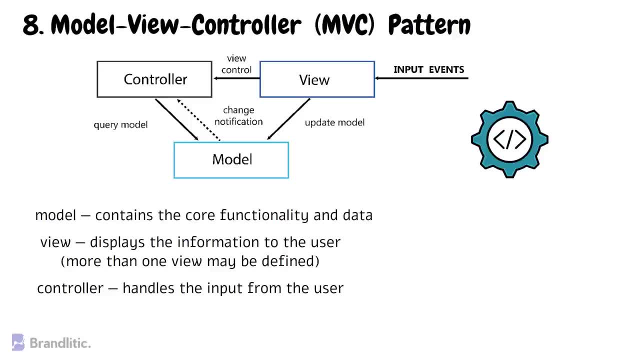 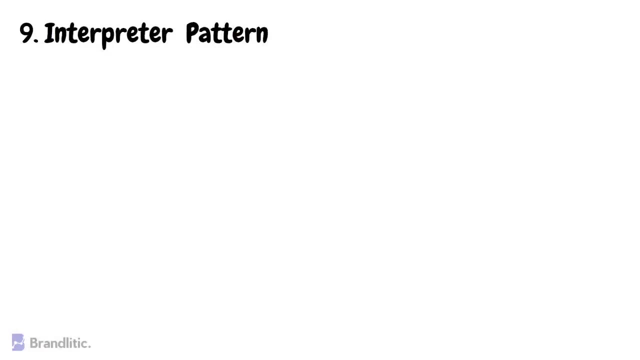 the user. It decouples components and allows efficient code reuse. This software architecture pattern forms as the foundation of web frameworks such as Django and Rails. 9. Interpreter Pattern. This pattern is used for designing a component that interprets programs written in a dedicated language. It mainly specifies how 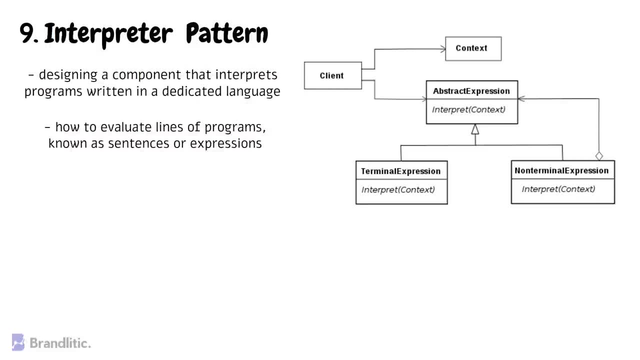 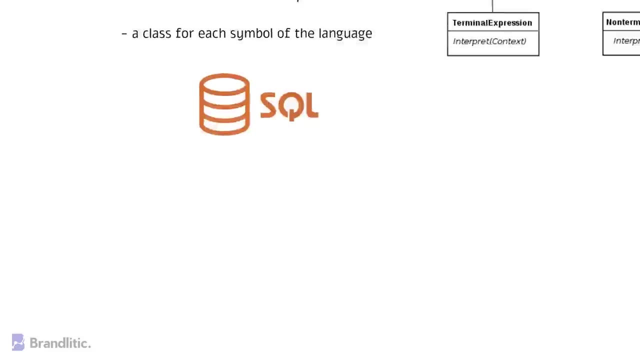 to evaluate lines of programs, known as sentences or expressions, written in a particular language. Here, the basic idea is to have a class for each symbol of the language. This software architecture is used in database query languages such as SQL 10.. Blackboard Pattern: This pattern is used for problems for which no. 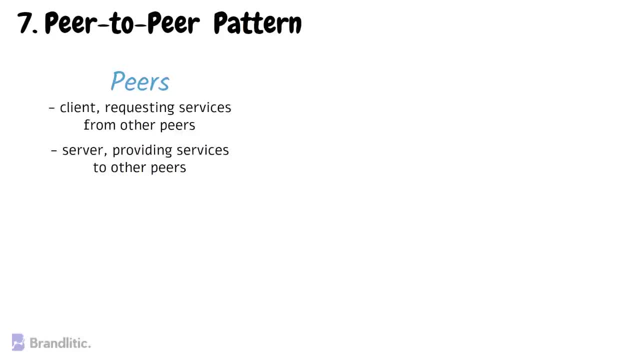 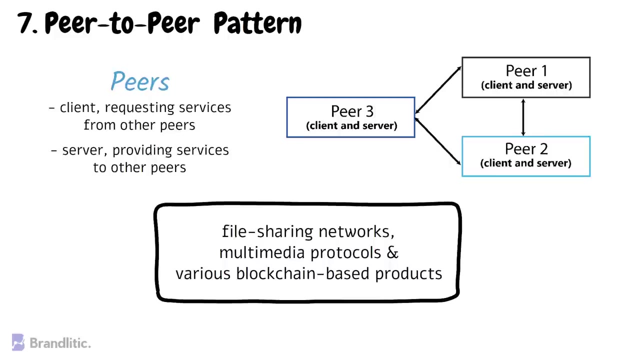 or as servers providing services to other peers. A peer may act as a client or as a server, or as both, and it can change its role dynamically with time. It is widely used in building file sharing networks, multimedia protocols and various blockchain-based products. 8. Model-view-controller pattern. 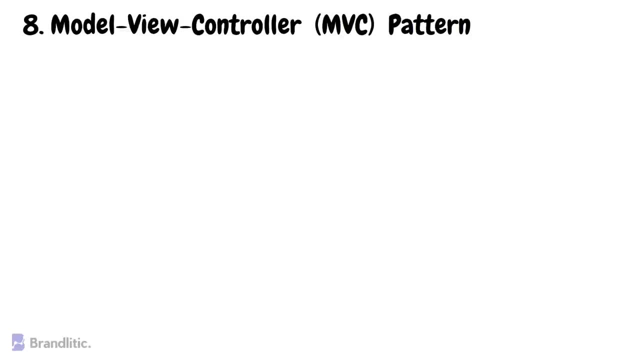 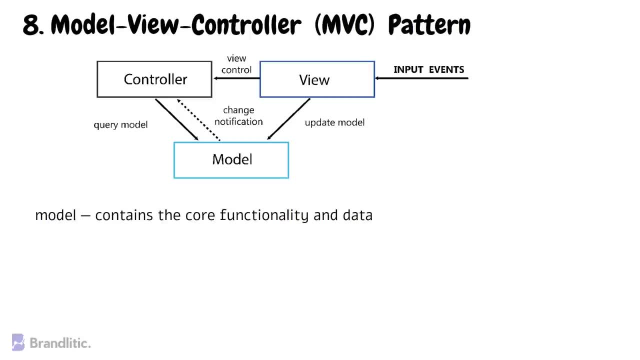 As: 1. Model, which contains the core functionality and data. 2. View, which displays the information to the user, and more than one view may be defined as well. 3. Controller, which handles the input from the user. This is done to separate internal representations of information. 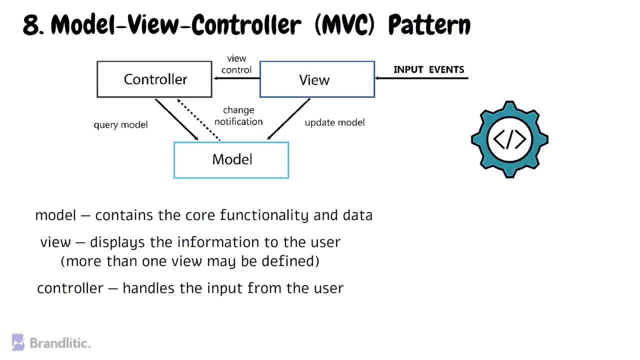 from the ways information is presented to and accepted from the user. It decouples components and allows efficient code reuse. This software architecture pattern forms as the foundation of web frameworks such as Django and Rails. forms as the foundation of web frameworks such as Django and Rails. 9. Interpreter pattern. 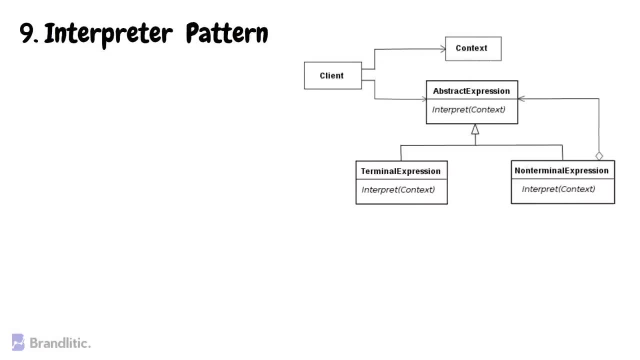 This pattern is used for designing a component that interprets programs written in a dedicated language. It mainly specifies how to evaluate lines of programs, known as sentences or expressions, written in a particular language. Here, the basic idea is to have a class for each symbol of the language. 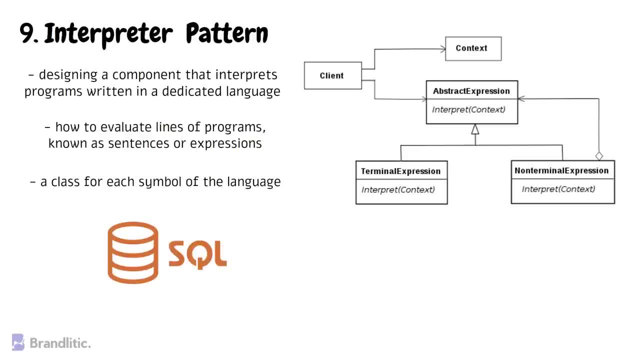 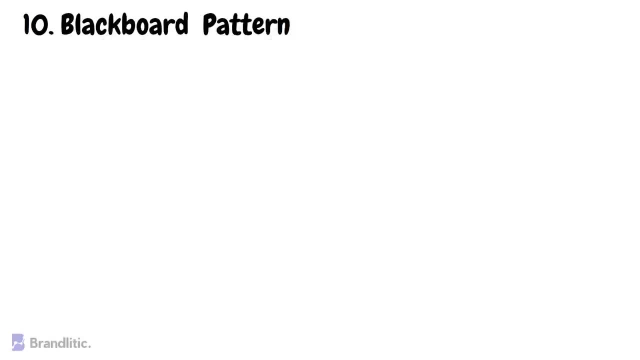 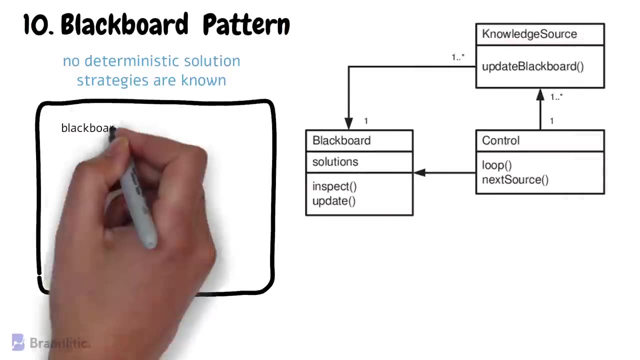 This software architecture is used in database query language. This software architecture is used in database query language. 10. Blackboard pattern. This pattern is used for problems for which no deterministic solution strategies are known. The blackboard pattern consists of three main components: 1. Blackboard, which is a structured global memory containing objects from the solution space. 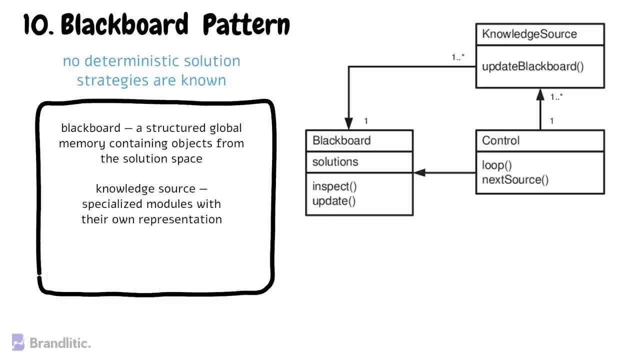 2. Knowledge source, which is specialized modules with their own representation. 3. Control component, which selects, configures and executes a specific module. 3. Control component, which selects, configures and executes a specific module. 4. Control component, which selects, configures and executes a specific module. 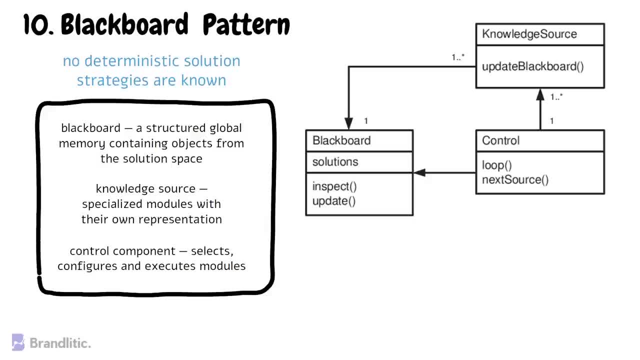 Here all the components have access to blackboard, and components may produce new data objects that are added to the same blackboard. Components look for particular kinds of data on the blackboard and may find these patterns matching with the existing knowledge source. This architectural pattern is widely used in applications that use speech recognition.